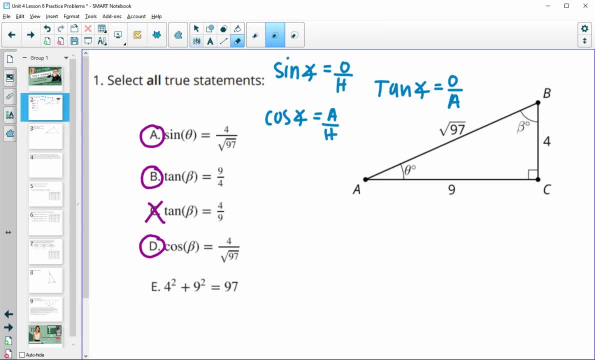 And then Part E is doing the Pythagorean theorem. So Part E says that we would do: 4 squared plus 9 squared equals 97.. And that is true, because 4 squared plus 9 squared should equal the square root of 97. 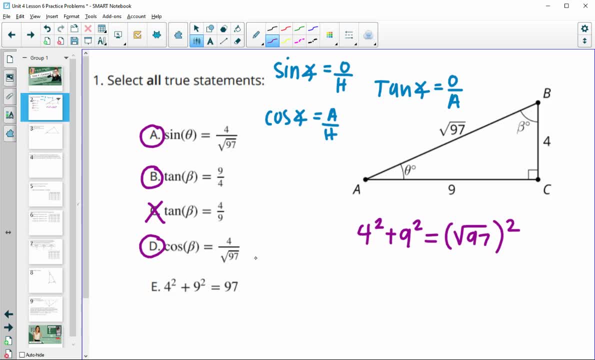 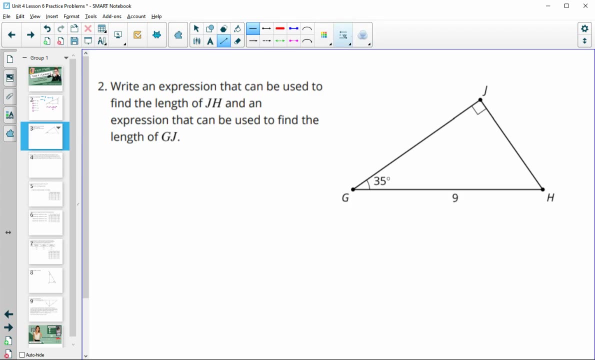 squared And the square root of 97 squared means that we would cancel the square root and the squared and that would just be 97. So E is correct as well. Number two: write an expression that can be used to find the length of JH. 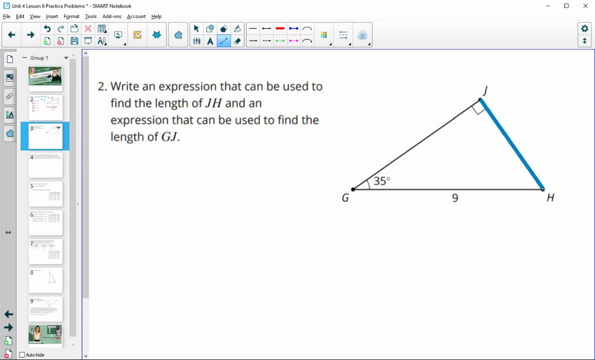 So here's JH and an expression that can be written to find the length of GJ There's going to be. there's multiple different ways that you can do this. I'm specifically going to use trig and I'm going to be looking at this 35 degree angle. 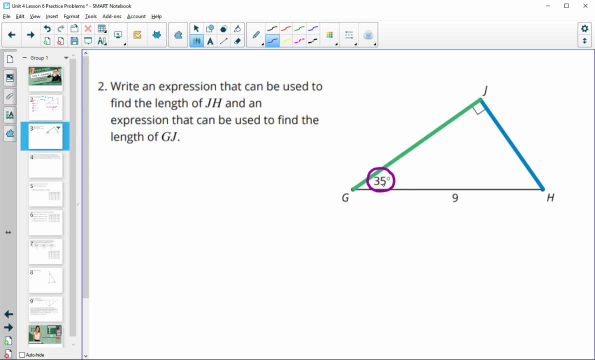 to label the sides. So for this, 35 across from the 35, so this blue segment would be the opposite side. The 9 is across from the 90, so the 9 is the hypotenuse, And so the green one is next. 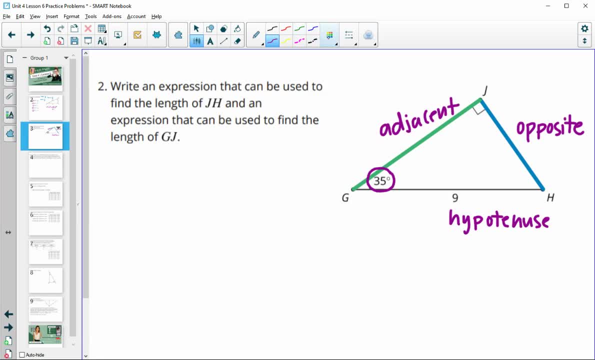 So I'm going to set up trig functions here. So for finding the opposite side. so I'm going to use the opposite and the hypotenuse, since I know the hypotenuse So opposite, and hypotenuse is a sine function. So sine of 35 equals the opposite side, JH over the hypotenuse 9.. 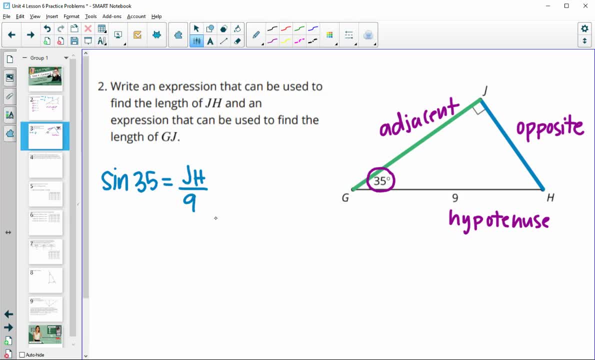 So there would be an expression that would help us, And you could just multiply the 9 up So it would be 9 times the sine of 35, would give us what JH is. Then to find the length of the green side, I would again use the hypotenuse and the adjacent. 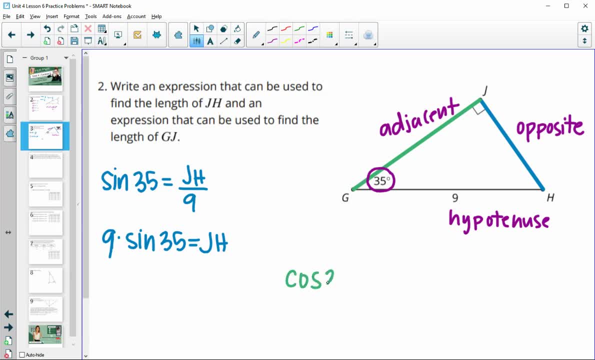 And that is a cosine function. So cosine of 35 would equal the adjacent side, which is JG, over the hypotenuse, Which is 9, so then I could multiply the 9 up and get that JG equals 9 times the cosine of 35.. 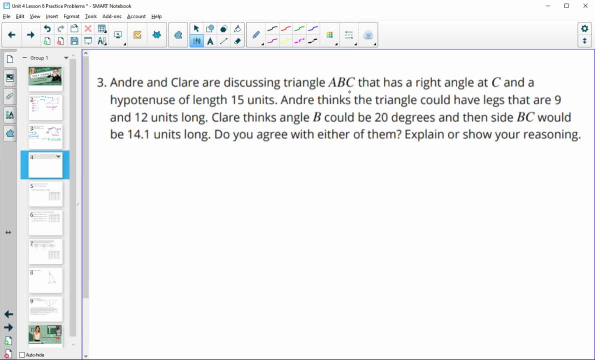 Number 3, Andre and Claire are discussing triangle ABC that has a right angle at C and a hypotenuse of 15.. So let's get that, So we know that the triangle that they're discussing, that angle C is the right angle and that the hypotenuse is 15.. 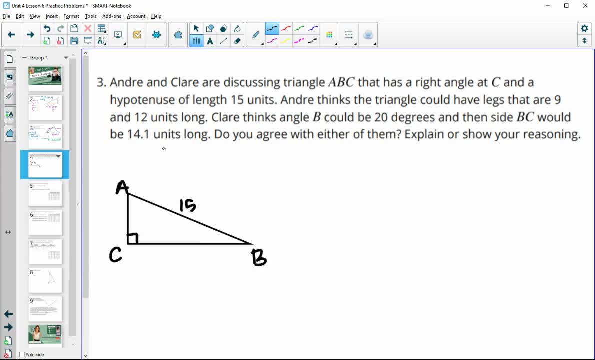 So it doesn't really matter where A and B go. Andre thinks that the triangle could have legs of 9 and 12.. So I'm going to do two triangles here, since we're going to have two different scenarios. So Andre thinks that they could have legs that are 9, that it could have legs that are 9 and 12.. 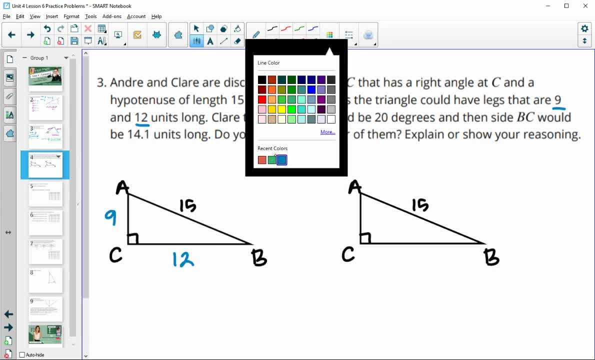 So I'm just going to put a 9 here and a 12 here, And then Claire thinks that angle B could be 20 degrees And then that side BC would be 14.1 units long. So do we agree with either of them? 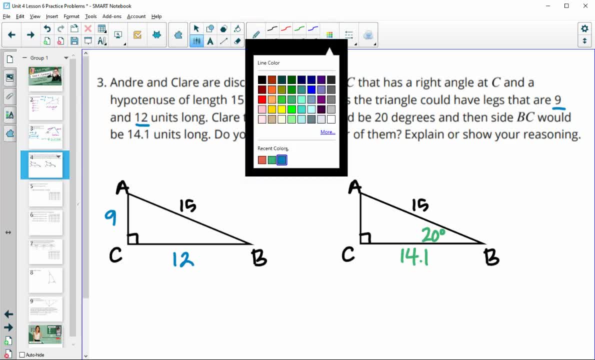 Explain or show the reasoning. So for Andre's, he just has all three. He just has all three sides labeled. So we could just check the Pythagorean theorem to see if this is in fact a right triangle. So 15 squared would need to equal 9 squared plus 12 squared. 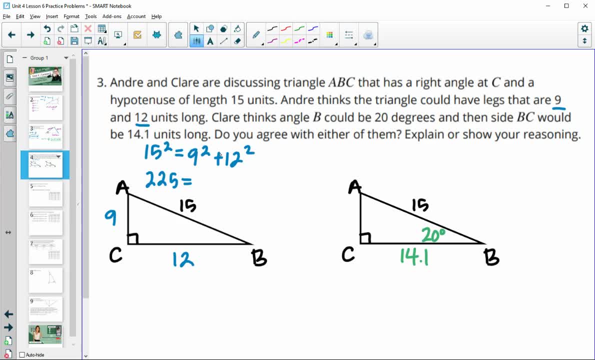 15 is 225. And then 9 squared is 81. And 12 squared is 144.. Those total up to 225.. So this is good. Okay, so a triangle certainly can Have side lengths of 9,, 12, and 15.. 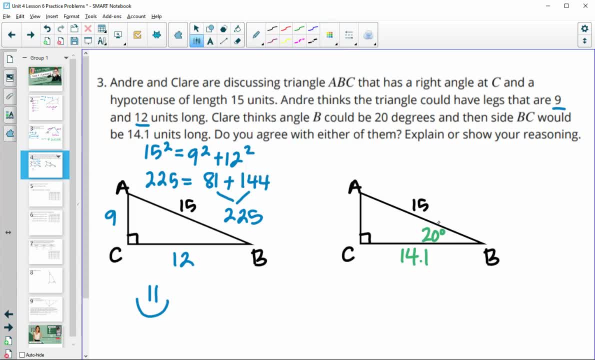 Then for Claire's idea. so Claire thinks that if this was a 20 degree angle, that this side would be 14.1, without hypotenuse of 15.. So for Claire's, we're going to be using trig to look at this. 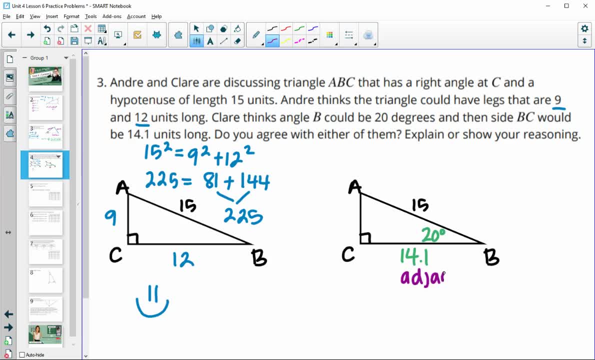 And so this 14.1 side is the adjacent side And the 15 is the hypotenuse. So we would be setting up a cosine function. So cosine of 20 equals the adjacent side, 14.1, over the hypotenuse of 15.. 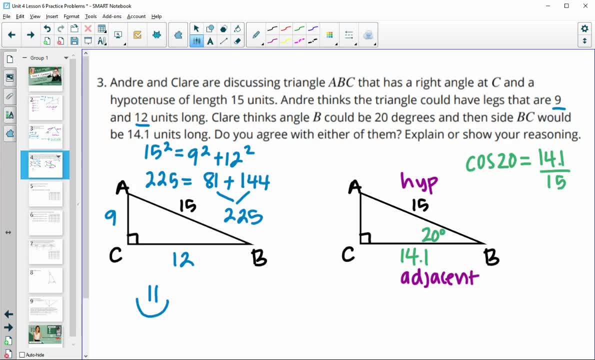 So we're just going to be looking to see that these all equal out. And if we put in the cosine of 20 into our calculator or look at it on our right triangle sheet, this equals 0.94.. And then we'll look at. 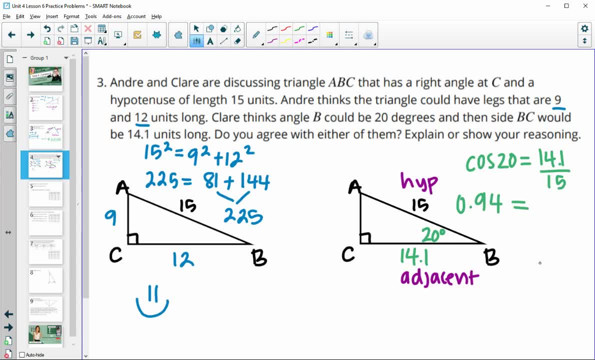 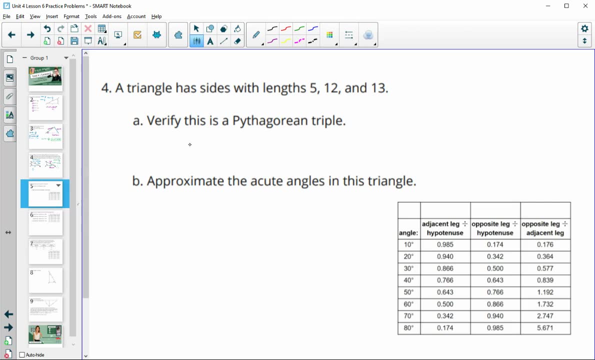 14.1 divided by 15.. And that also equals 0.94.. So this information can work together as well, So they're both right. Number four triangle has sides of 5,, 12, and 13.. Let's verify that. it's a Pythagorean triple. 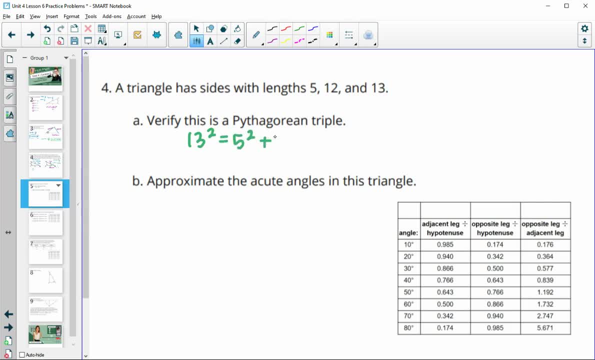 So we will put this into the Pythagorean theorem and see that both sides equal: 13 squared is 169.. 5 squared is 25.. And 12 squared is 144.. 25 plus 144 is 169.. So this is good. 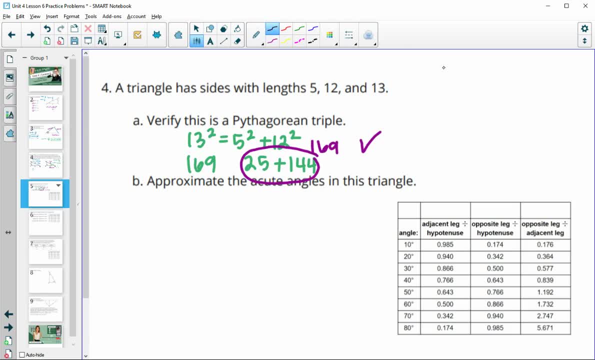 Then we want to approximate the right angles in this, Or sorry, the acute angles in this triangle. So if we kind of draw this triangle, we've got legs of 5 and 12 and then a hypotenuse of 13. So if I go ahead and just pick an angle to find right away, 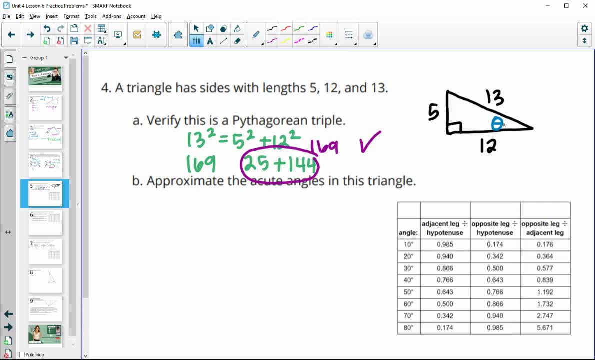 So I'm just going to go ahead and do that. I'm just going to find this one. So this one, the 5.. You can use any side you want. I'm going to use the 5,, which is the opposite. 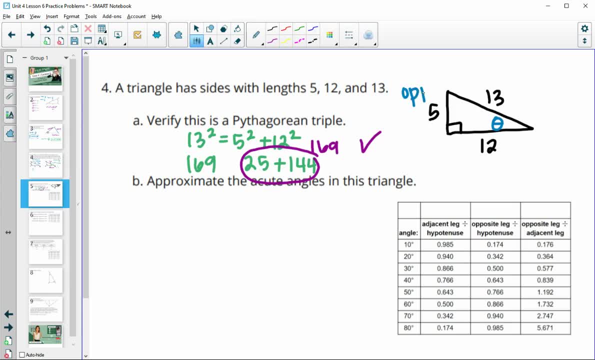 Because it's directly across from the angle. So this is the opposite side, Next to it is the adjacent side. So I'm going to be looking at opposite over adjacent, which is this final column here. So 5 divided by 12.. 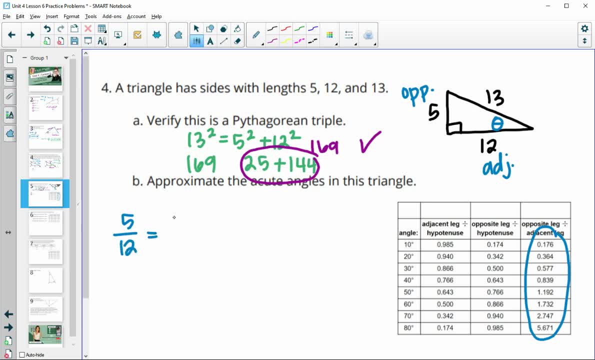 If we do that In our calculator, we get a decimal of 0.416 repeating. So then let's look in this column of opposite divided by adjacent, to see where we get the closest. So we can see it's between these two numbers. 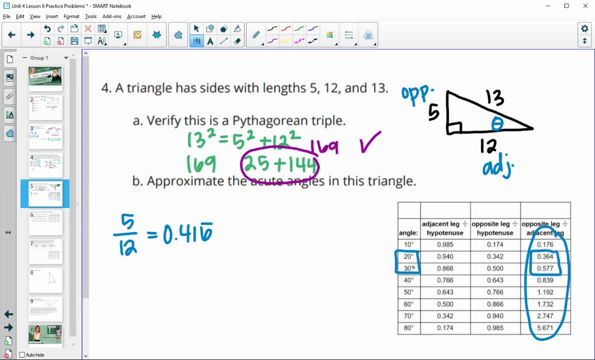 So that angle is somewhere between 20 and 30. And it's a bit closer to the 0.36. So it's a bit closer to 20.. So maybe We would say that that means that theta or that angle is maybe about 23 degrees. 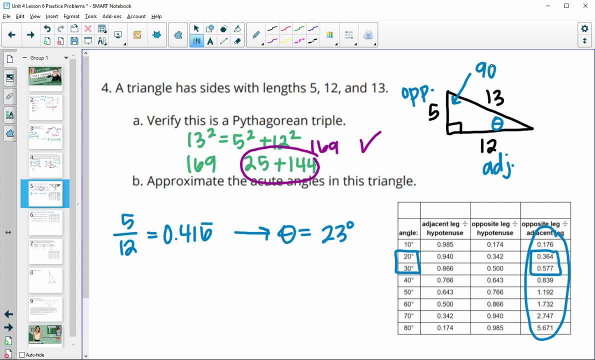 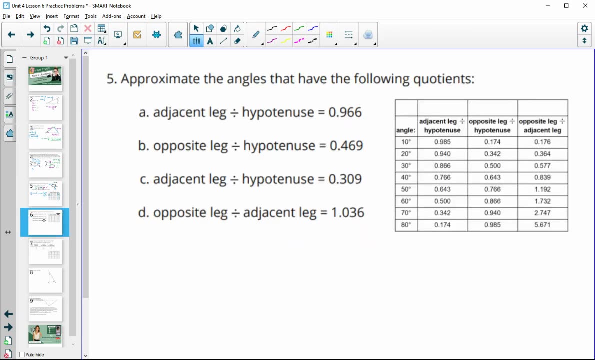 And then we know that this one would just be 90 minus whatever theta is, So we could do 90 minus 23. And we could get 67 for the possible other angle Number five approximate: Approximate the angles that have the following: 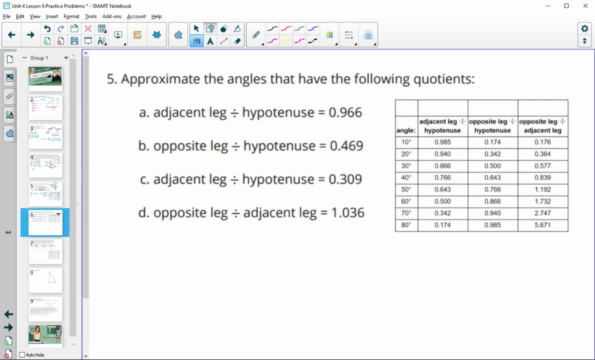 Quotients. So we're going to take a look in this table at the ratios they're giving us. So for this first one they're doing adjacent divided by hypotenuse. So that's in this first column And we're looking for where 0.966 would land. 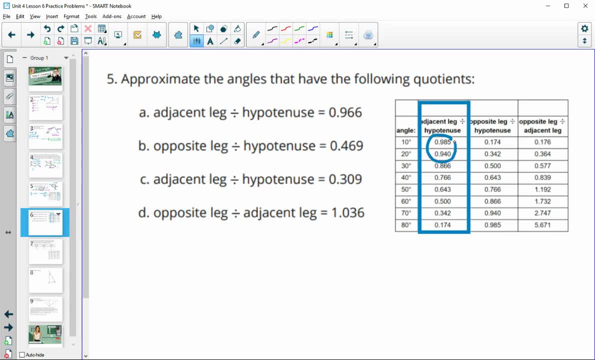 So 0.966 is going to be somewhere between these two numbers And looks like about halfway in between, So between 10 and 15 or 10 and 20 degrees, So I'm going to say about 15.. The next one is the opposite divided by the hypotenuse. 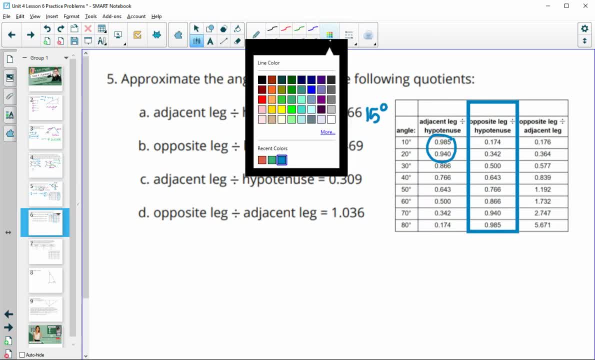 So now we're looking in the middle column for where the decimal point 469 fits, And so 469 is going to fit somewhere between here And maybe a bit closer to 0.5.. So maybe, and so between 20 and 30.. 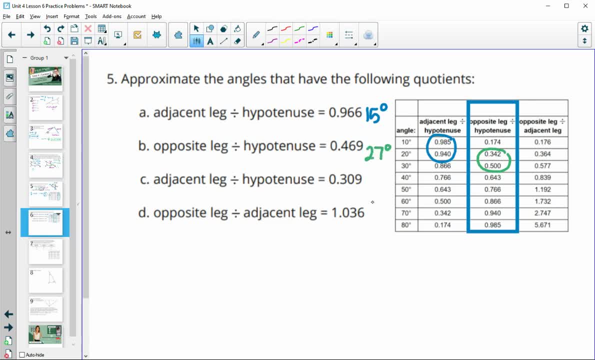 So maybe 27 degrees, Next one adjacent over hypotenuse again. So now we're in this first column And it says 0.309.. So 0.309 is somewhere between 0.17 and 0.34.. 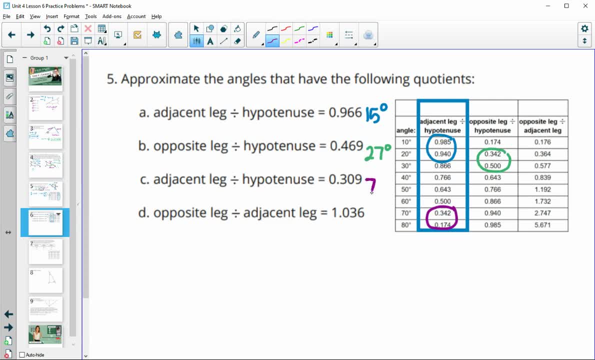 Closer to 0.34.. So closer to 70. So maybe like 72 or 70. Or 73 degrees, And then the final one is the opposite divided by the adjacent. So that's this final column, And this one has us looking for the ratio of 1.03.. 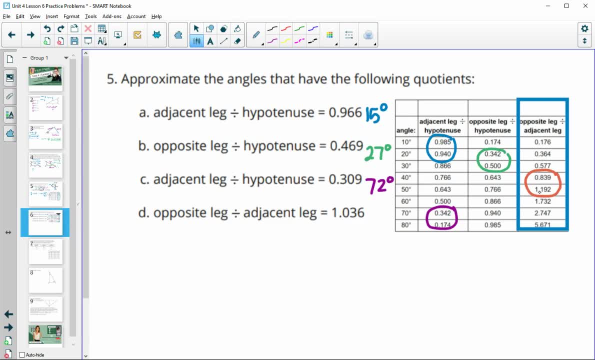 So 1.03 is between 0.8 and 1.2. And it's probably maybe about halfway in between or so, And so maybe around 4.3. Or 4.5.. 44,, 45, something like that. degrees. 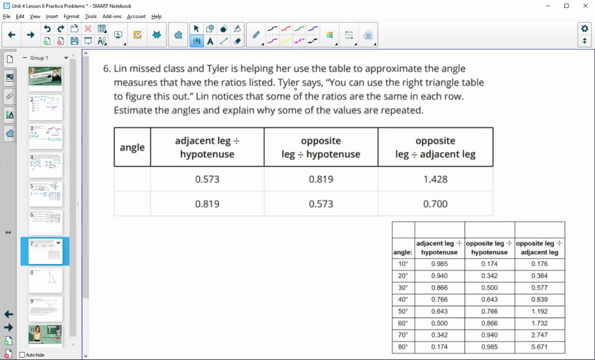 Number six: Lynn missed class And Tyler's trying to help her use the table to approximate the angle measures that have the ratios listed. Tyler says you can use the right triangle table to figure this out And Lynn is noticing that some of the ratios are the same in each row. 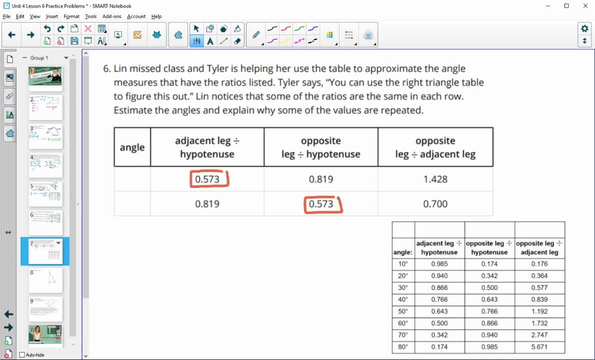 So noticing that this one is the same as this one, And then also that this one is the same as this one. So now estimate the angles. So we know, if these kind of the cosine ratio and the sine ratio flip, that the angles right here are going to total 90 degrees together. 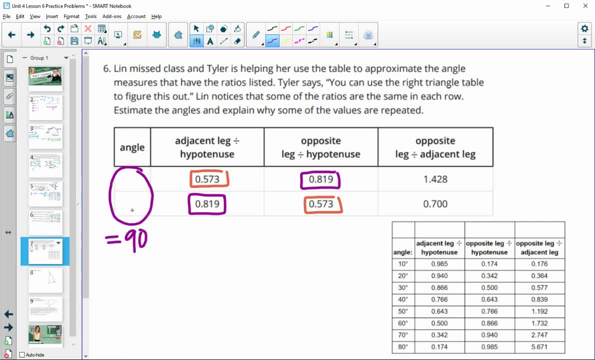 So if we just approximate one, we can kind of just know what the other is by subtracting from 90.. So let's take a look at the table and look at the adjacent over hypotenuse for 0.57.. So adjacent over hypotenuse for 0.57 is going to be between, here, about halfway between: 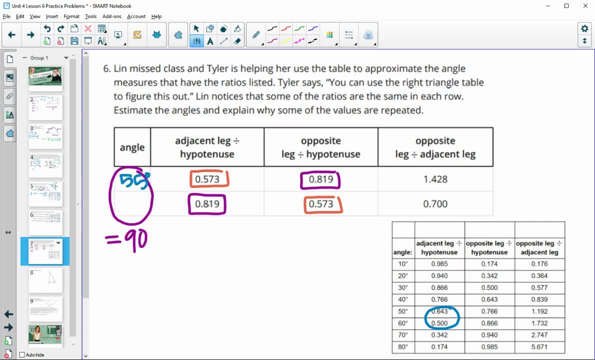 So about 55 degrees. So again, you can then go and look for this 0.82 if you want to, Or you can do 90 minus 55 and get 35. for a good estimate for that next one, Number seven: find the length of each leg. 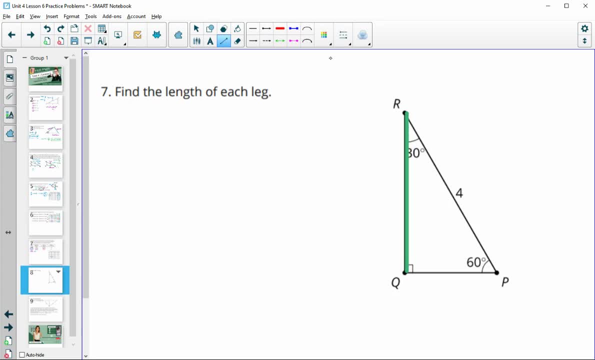 So we need to find our Q and then we also need to find PQ. Now you can use trig in this, because you have angles. You can also see that this is a 30-60-90 triangle. So remember from our 30-60-90s that the hypotenuse, this short leg, is half the hypotenuse. 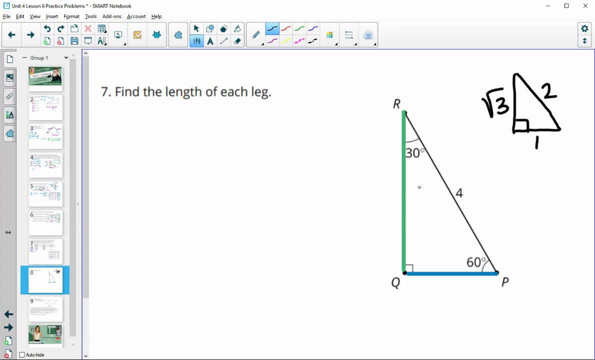 And then the long leg is the short leg time. The short leg times the square root of three. So I'm just going to do that because I find that to be quicker. So we have: the hypotenuse is four. So this short leg across from the 30 is going to be half of that four. 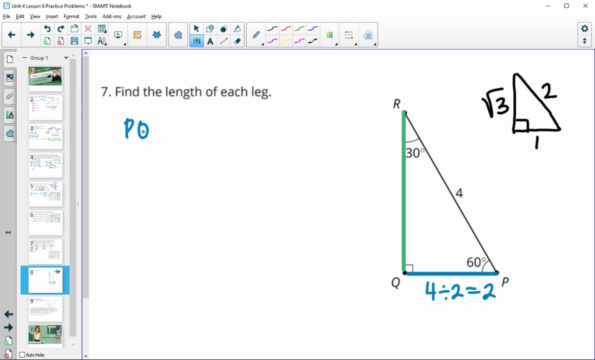 So four divided by two is two, So PQ is equal to two. Then for the longer leg, or the one across from the 60, it's going to be the short leg times the square root of three. So then this is going to be two times the square root of three. 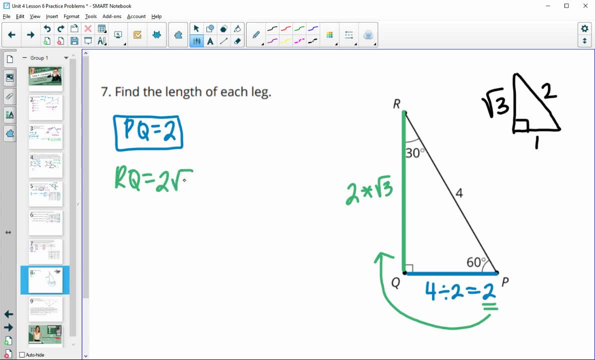 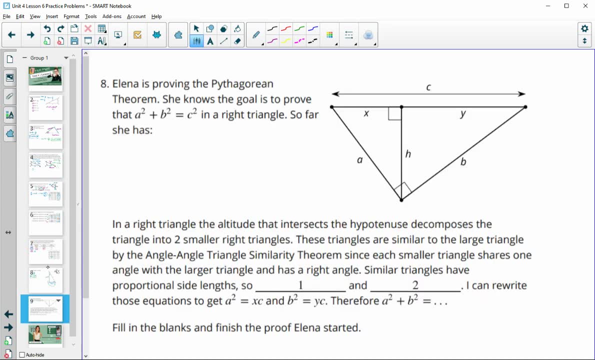 So our Q is equal to two square root of three. Number eight says Elena is trying to prove the Pythagorean theorem. She knows the goal is to prove that A squared plus B squared equals C squared in a right triangle. So far she has done this. 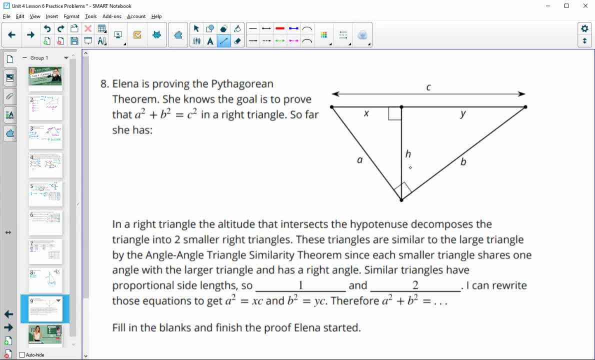 So she knows that in a right triangle the altitude intersects. When the altitude intersects the hypotenuse, it decomposes it into two smaller right triangles. These triangles are similar to the large triangle by angle angle, Since each smaller triangle shares one angle with the larger triangle and has an acute angle. 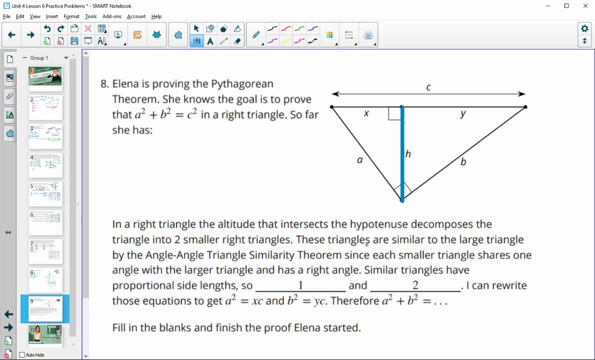 So similar triangles have proportional side lengths. So then, what does she know? So proportional side lengths, we're trying to write in a proportion here. I'm just going to write it up here so that we can Look at it a little bit easier. 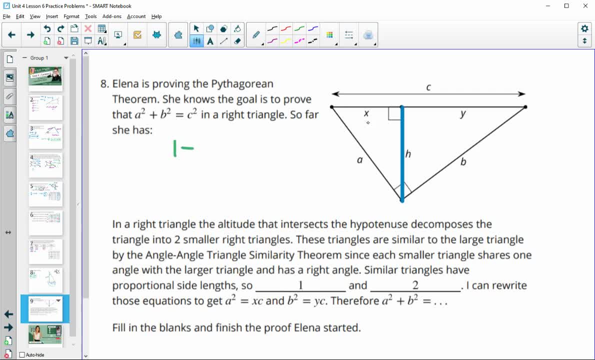 So one she's going to write something with this little triangle to the big triangle And so for this one she could say that this short leg over the hypotenuse, So X over A in the smaller triangle, equals the short leg over the hypotenuse in the big triangle. 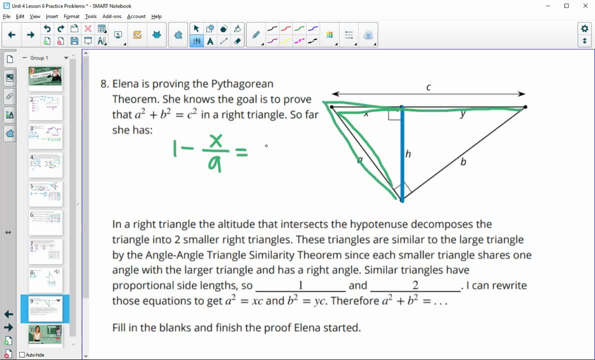 So short leg over hypotenuse in the big triangle, So A over C, And then for number two she's going to do a similar thing with the other triangle. So now she's got in this triangle, she's got the longer leg over the hypotenuse she could do. 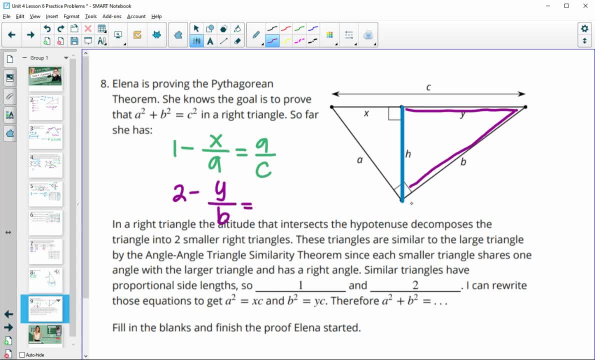 So she could do Y over B And that's going to equal the longer leg over the hypotenuse. OK, so B over C For that bigger triangle. This is going to get her both A and A twice and B twice in her proportions. 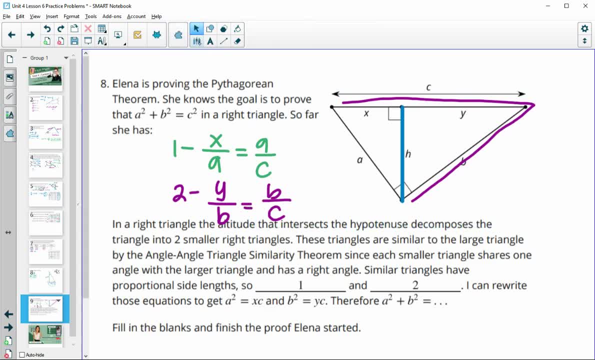 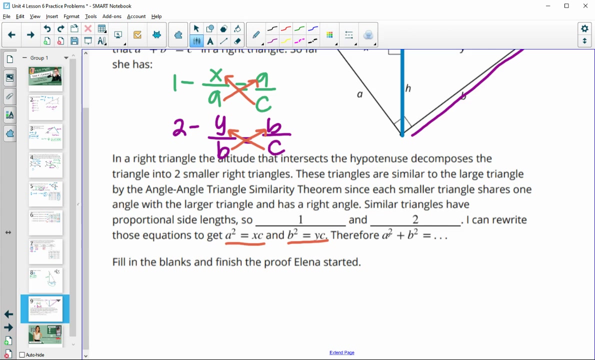 Which will help her to get this, because then if she cross multiplies here, She would have A squared And X times C, which you see that she has here. So A squared equals X times C, B squared equals Y times C. So that helps her because therefore A squared plus B squared.